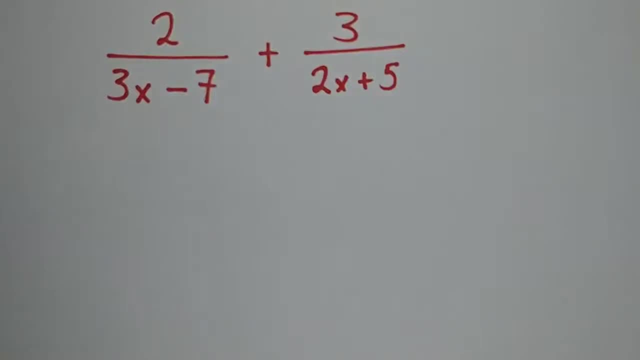 So in this video we're going to look at how to add or subtract two fractions to make them as a single fraction. So what we need to do is we need to find the lowest common multiple. So now the LCM in this case is just the product of the denominators. 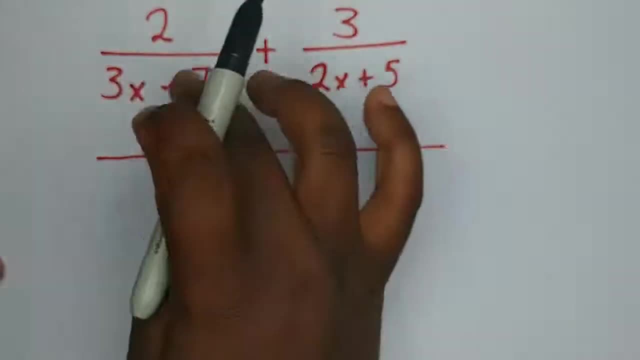 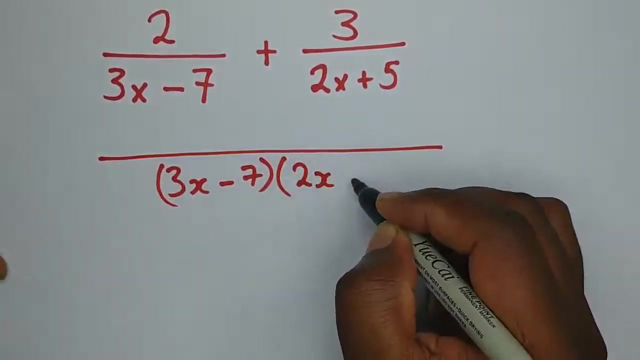 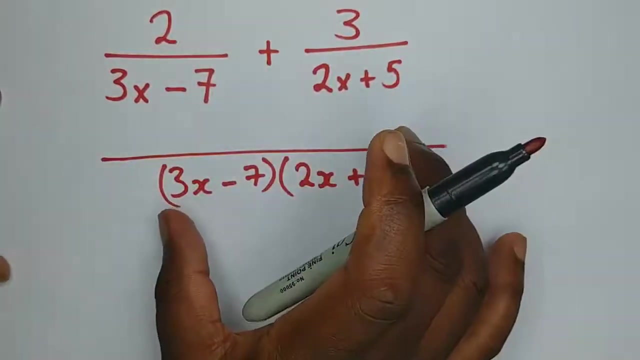 So this is what we mean: The product of the denominators, which is 3x-7 and 2x-5.. This is the product of the denominators. Then what we're going to do is this denominator, if it goes into the product of the denominators, we're going to get the opposite. 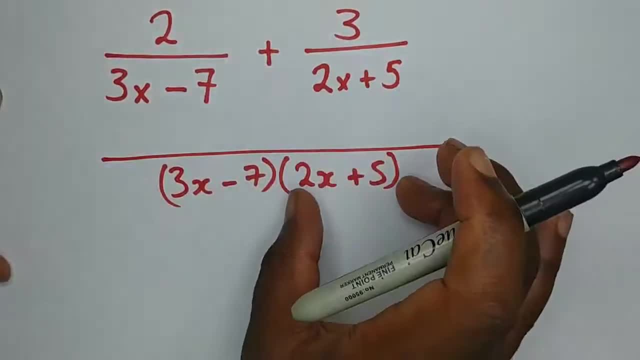 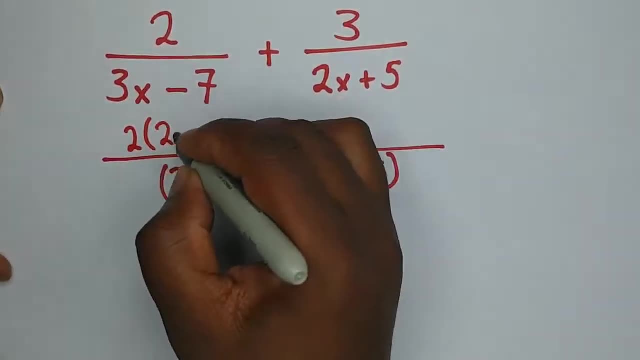 So this one and this one will cancel. So if this goes into this, we're going to get this guy. This will multiply the numerator, So we'll have 2, the numerator multiplied by this, which is 2x plus 5.. 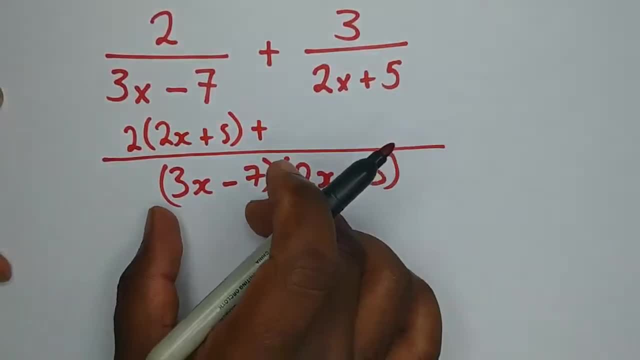 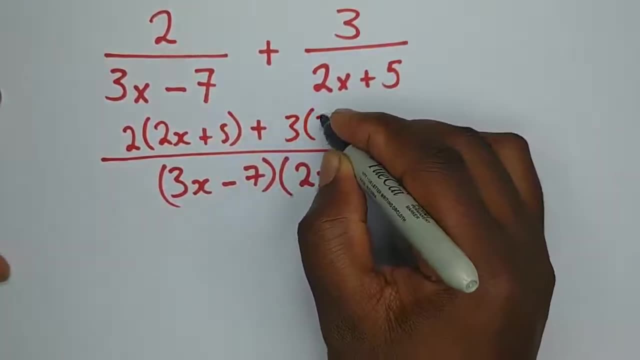 Plus, if this goes into this, what we're going to get is the other denominator, which is 3x-7.. 3x-7 will multiply with 3x 3 to give us 3.. 3x-7, like that. 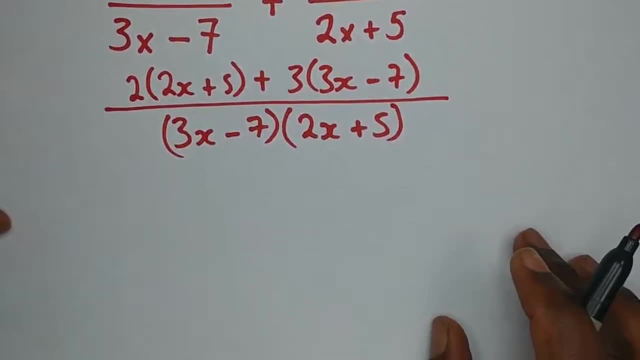 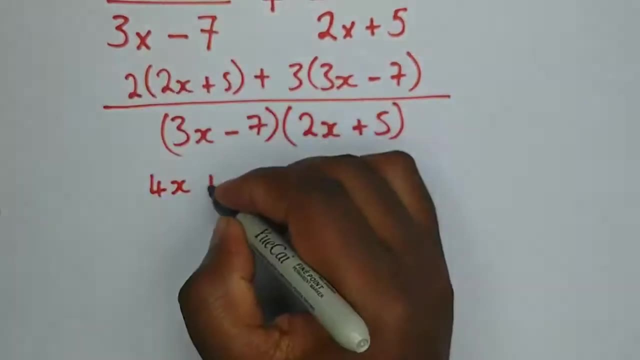 Then all we need to do now is to expand the numerator. So, expanding the numerator, what we're going to get will be 2 times 2x, we get 4x, 2 times 5, we're going to get 10.. 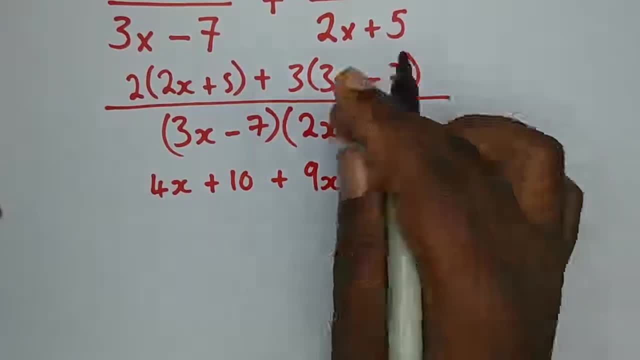 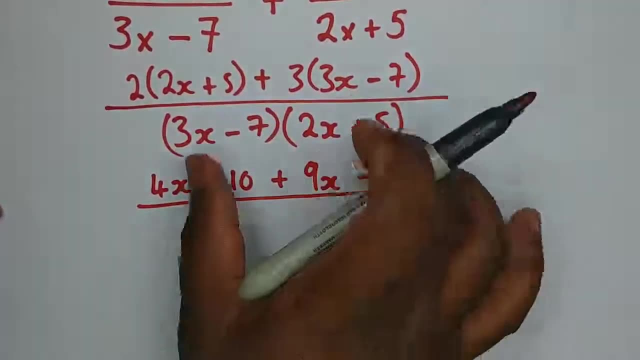 Plus 3 times 3x, we're going to get 9x. 3 times 7,, we're going to get negative 21.. Now, remember, we still have the same denominator, which is this one here. No need of expanding it. 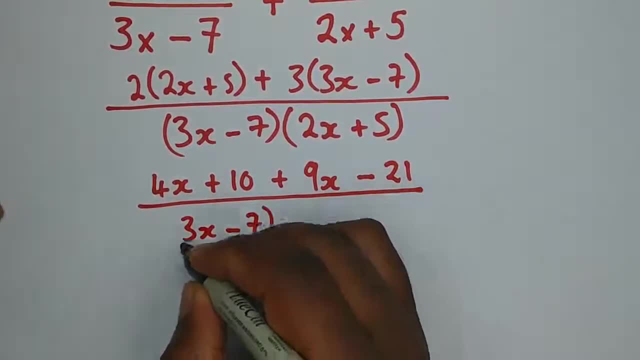 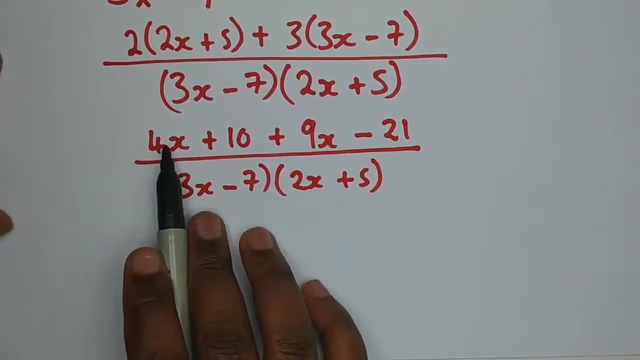 As it is like that: 2x plus 5.. So we're just going to add like terms now, The like terms being 4x and 9x. So 4x plus 9x will give us 18x. 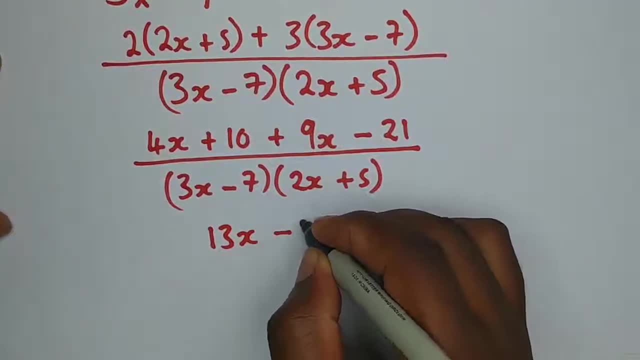 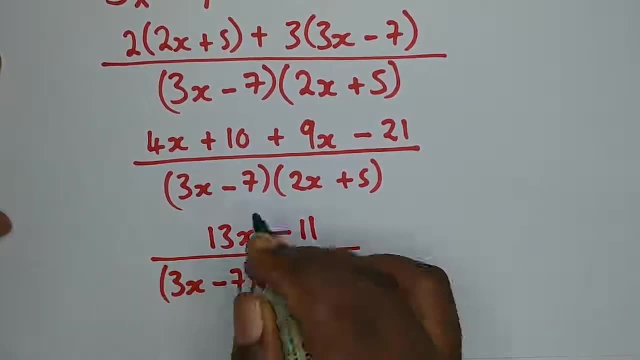 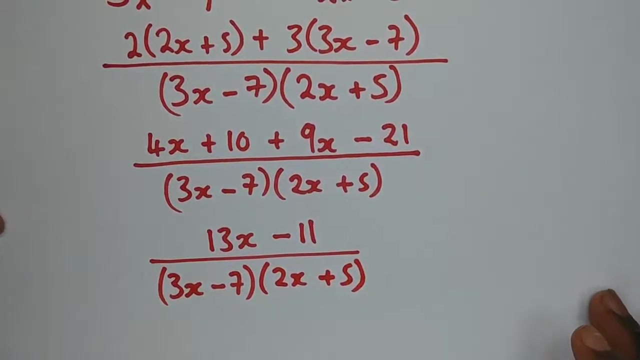 10 minus 21 will give us negative 11.. And all this is over 3x minus 7, which is our common denominator- multiplied by 2x. So we have made the fraction as a single fraction. Okay, let's look at one more example. 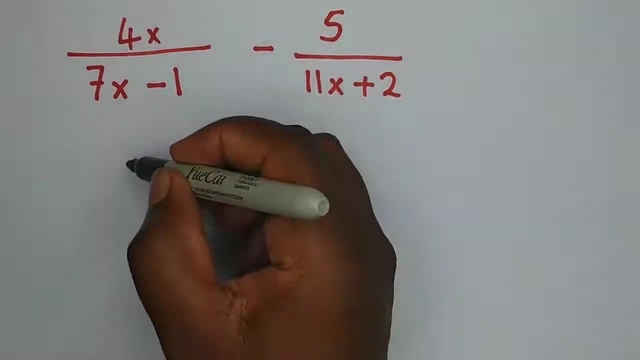 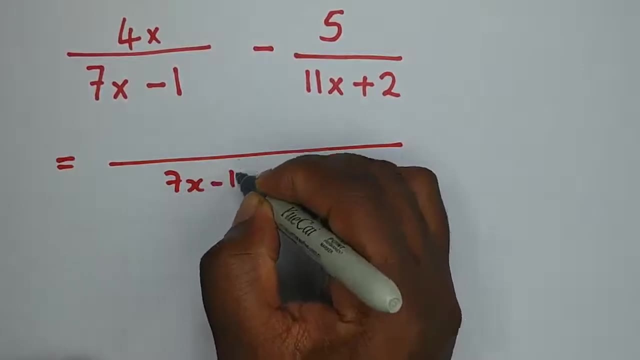 Okay, so the same concept is applied here. We're going to find the LCM. Now, the LCM is just a product of the two, So our LCM will be 7x minus 1, multiplied by 11x plus 2..